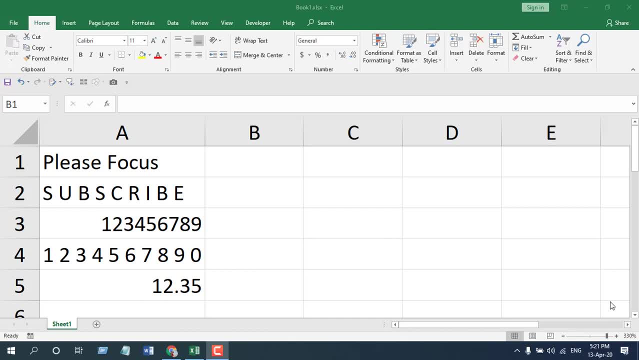 How to use the substitute function in Microsoft Excel. Hello everyone, welcome to Excel 10 tutorial. In this function explained video series, I'm going to explain you the substitute function. okay, I'm going to talk about the parameters and I'm going to talk about how you should use it. what is the? 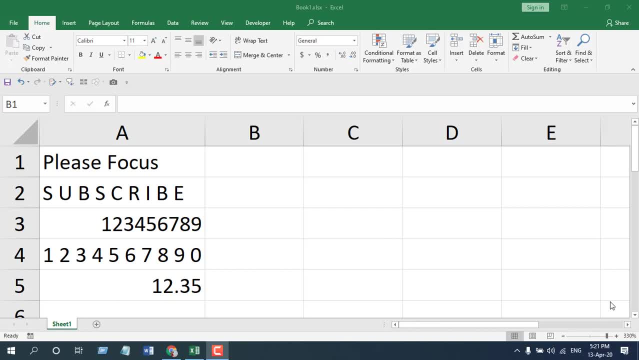 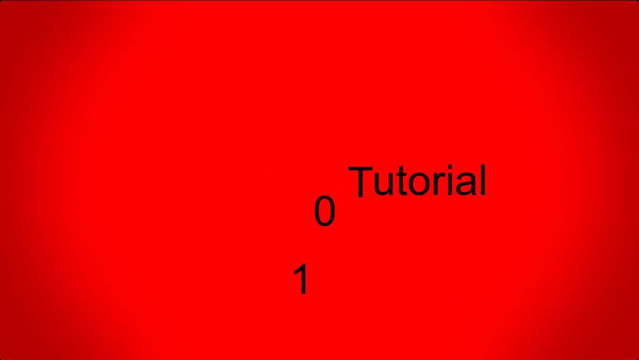 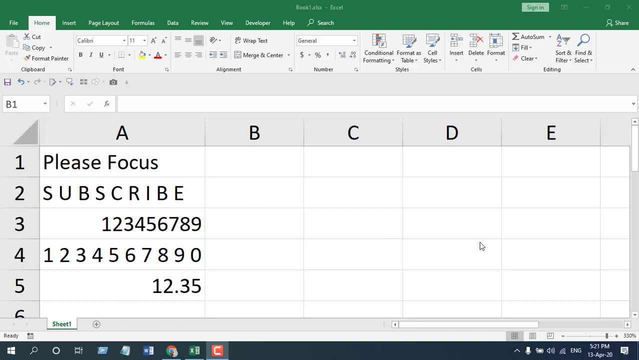 reason behind this function and what is the best way to use this function? okay, So let's get started. I think the best way to learn a function is to apply it, and we are going to learn how to use substitute function by simply applying. okay, So let's apply it here. First, we'll have to write. 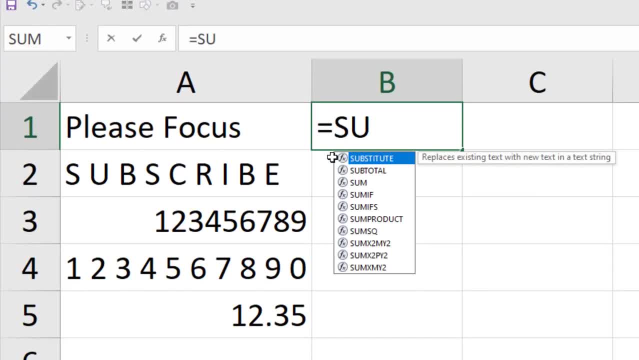 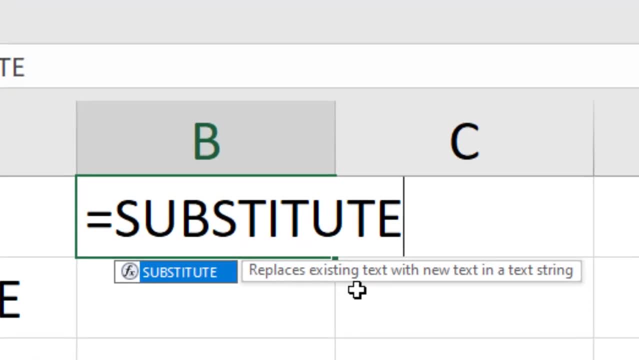 equal and then we'll have to write su and you can see here substitute. this is our function today. So this is the substitute function and you can see here: replaces existing text with new text in a text string. Okay, That means substitute function is used to replace certain text with a new text inside. 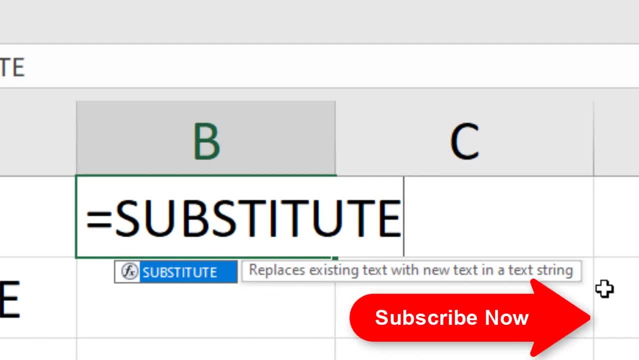 a text string. Okay, So this is why substitute function is used and this is why you should use it. If you need to replace text inside a text string, you can use substitute function. Okay, So give it open parenthesis. and here is the parameters of substitute function. The first one: 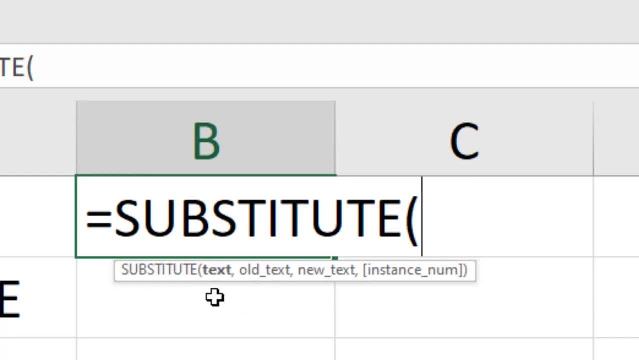 is text, So in which text you want to replace, you will have to select it here. and the next parameter is all text. That means the text string you are going to replace. and then the third parameter is new text. That means the new text you are going to replace. three and the last parameter is instance number. 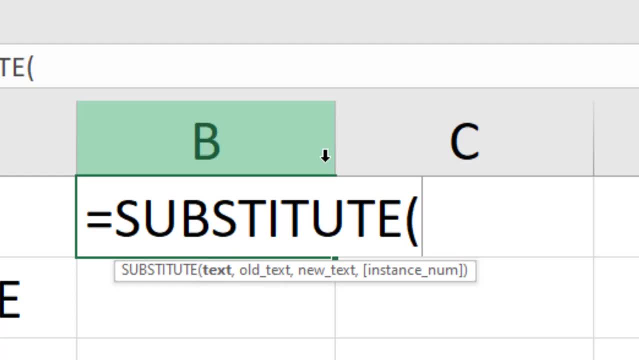 That means, if you have that text in your data range three times, so which one you are going to replace. The first one? if it's the first one, that means the instant number is one. If it's the second one, then the instant number is two, and if it's the third one, the instance number will be three. 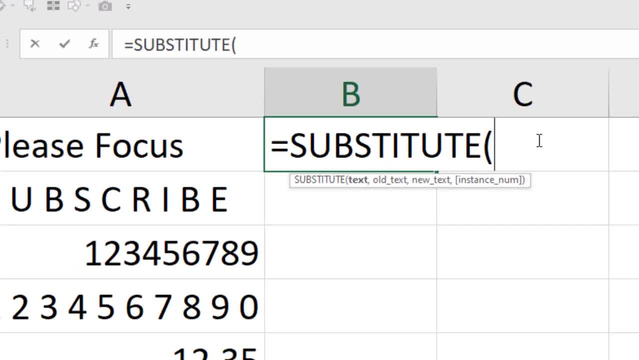 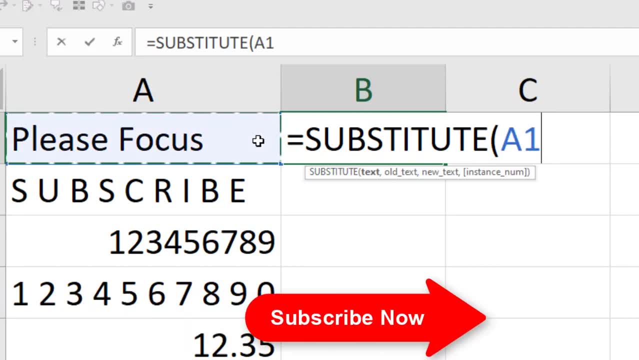 and so on. Okay, So let's start Start our function here. So first we are going to select the text. You can write the text here, or you can select the cell number or data range where you have the text. Okay, So this is our. 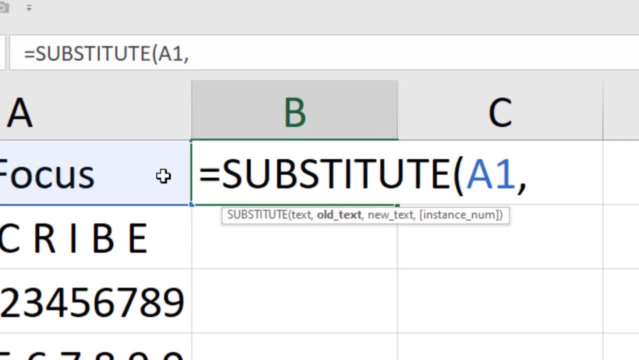 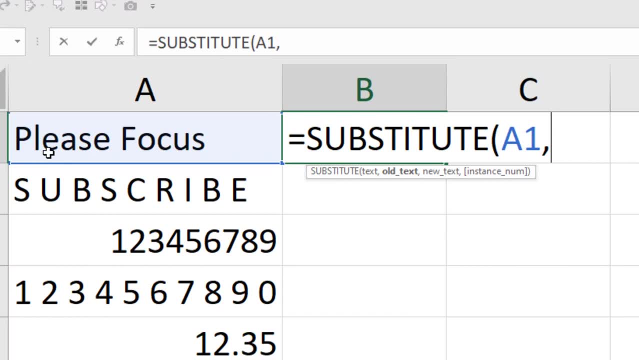 first parameter and if I press comma, you can see we just move to the next parameter, which is the old text. Okay, So we are going to remove the character e here. Okay, Which is in a small letter, and we have two occurrences of this character in this selected range. Okay, So let's write e inside. 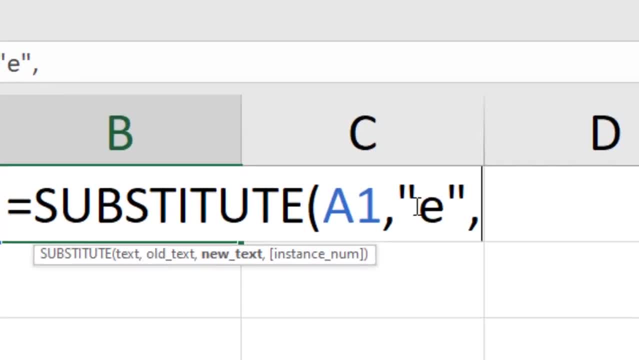 here. Okay, Now, if we added a comma, we are going to move to the next parameter, which is the new text, and we are going to replace the character e with capital b. Okay, And now, if I put another comma here, we are moved to the next parameter, which is the instance number, and there are two. 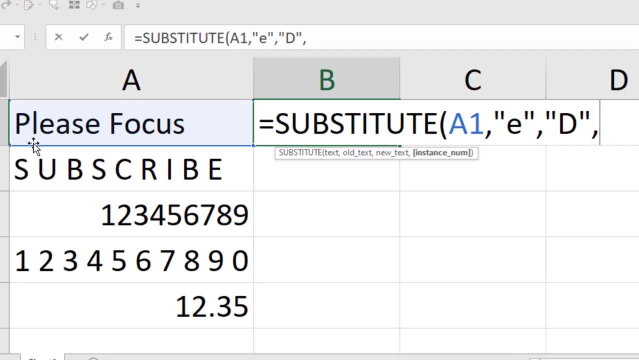 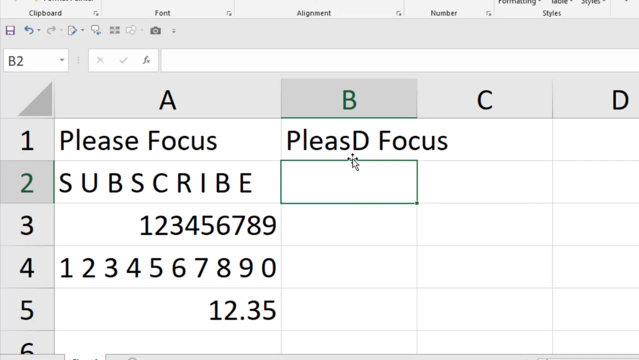 occurrence of this character here, e, here and here. So we are going to replace only the second occurrence of this character. Okay, So if I give it two and close parenthesis and press enter, you can see we have changed the character e with the new character capital d. But here is the important. 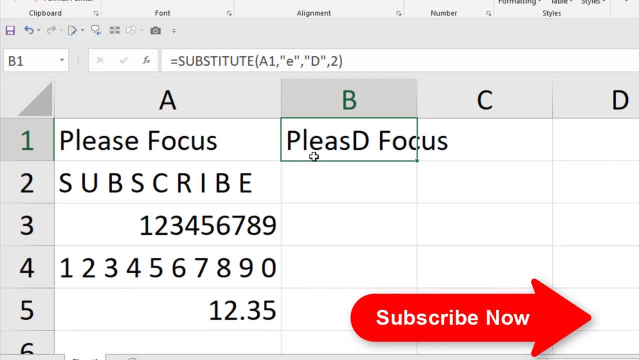 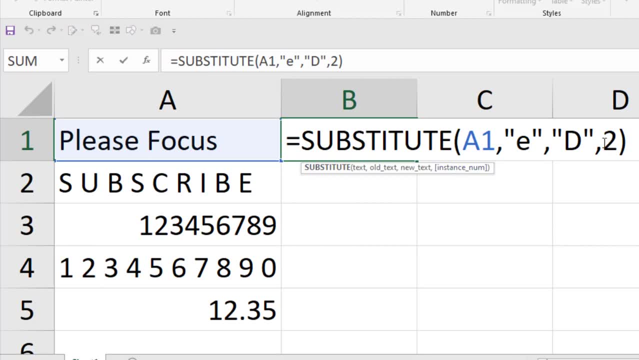 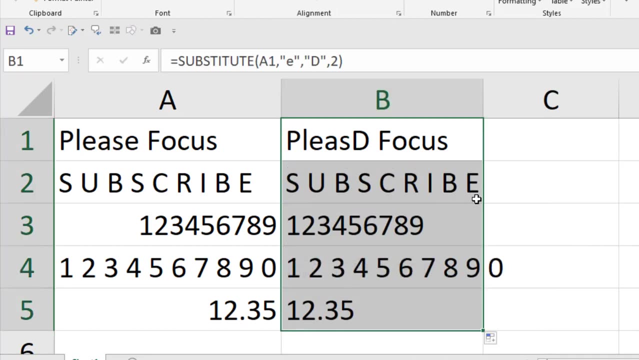 part. We had another e here, but it didn't replace this because we had selected the second instance number. You can see it here. Okay, So instance number was two. that's why we replaced only the second instance. Okay, Let's drag it Now here. we have only one e here and this is why it didn't. 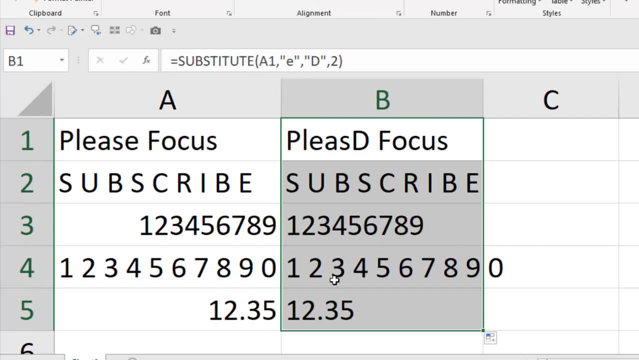 replace it and in this range we don't have that specific character. That's why we don't have that one, That's why nothing has changed. So I hope you understand. the substitute function has been explained. So you have four parameter here: The main text, the text you want to replace, the text. 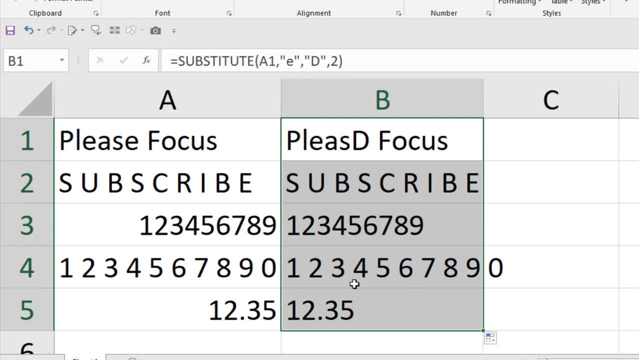 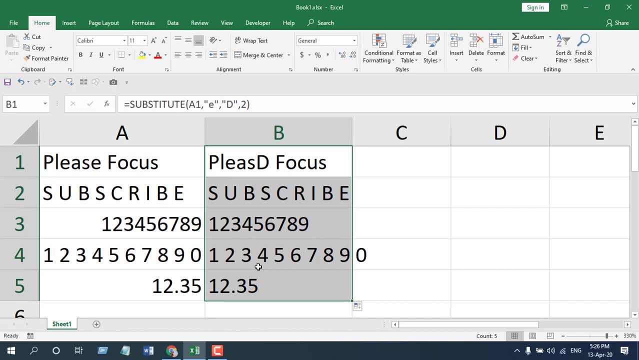 you are going to replace with, and the last one is instance number. Okay, So this is how you can use the substitute function in Microsoft Excel. If you like this video series, please let me know. I'm going to explain a lot of function in this series and please subscribe to the channel for future. 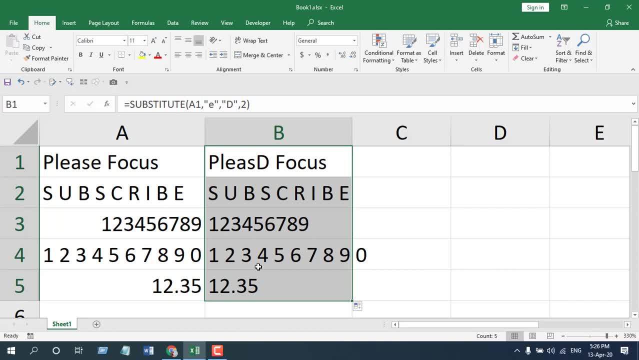 videos. If you can, please share this video with your friends and family. Thank you very much And, if it's possible for you, please support the channel through Patreon. Thank you, Thanks for watching. See you in the next tutorial. Don't forget to subscribe. Thank you.